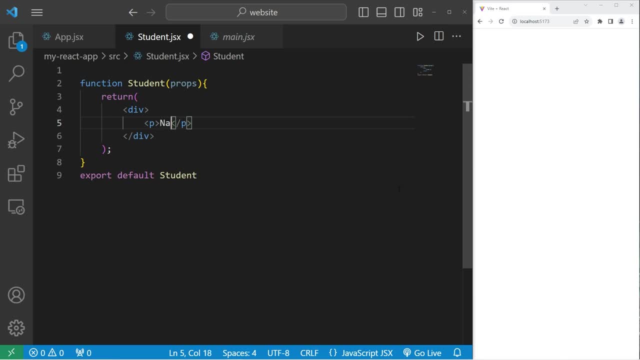 paragraph element. Within our paragraph we'll add the text name colon space. We'll include a set of curly braces to inject some JavaScript. Let's take our props. this is an object: access the name property. However, we still need to pass in a value for the key name. So, heading back to 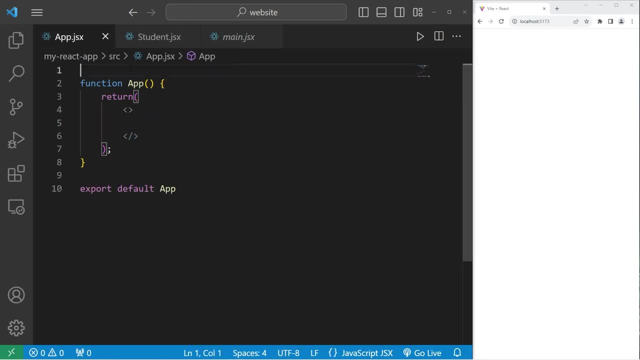 our app component. we need to import the student component. Let's do so at the top: Import student from the location where the student file is found: Dot forward slash, student, dot jsx. Let's include a student component within our app component: Student. Now, if I would like to send some data to my student component, student is going to be the. 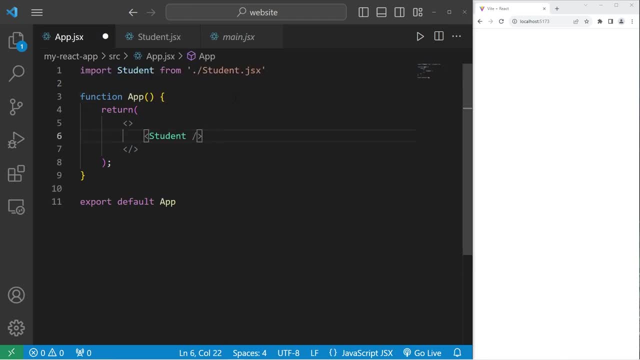 child- in this case, App is the parent. We'll need to list key value pairs. The key will be: name equals some value For the value associated with the name key. let's say Spongebob. When I save and update everything, we have the name Spongebob When we send key value pairs. 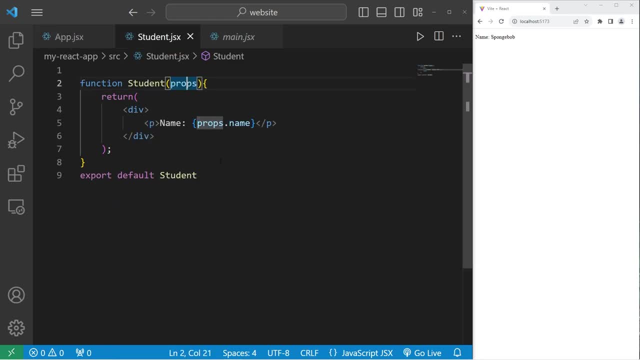 to a component. they're all stored within this props object. To get the value associated with the key, you type props dot- the name of the key. That will give you the associated value. On my web page I'm going to zoom in a little bit just so you can see it. That's good for now. 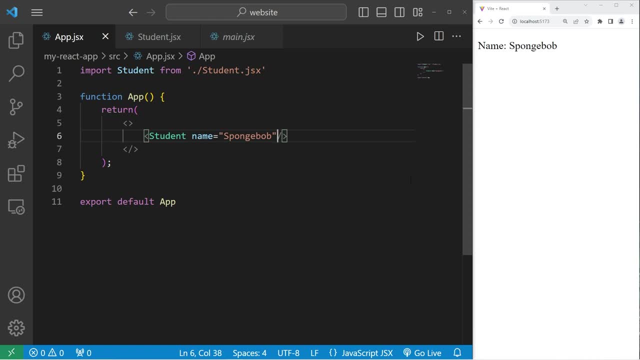 Heading back to our app component, let's send another key value pair. Let's send an age. If you're going to store some data as a value, if it's not a string literal, you got to enclose it within curly braces. Let's say, Spongebob: If you're going to store some data as a value, if it's not a string literal, you got to enclose it within curly braces. 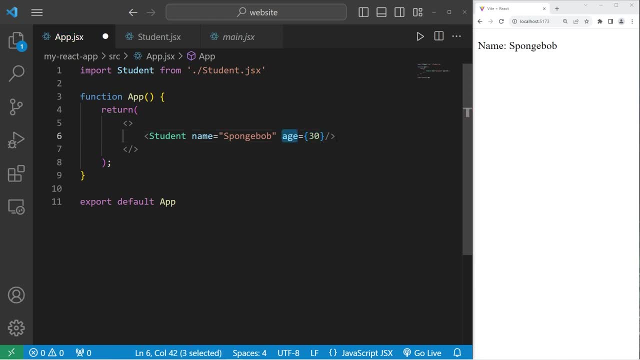 Spongebob. his age is 30. We now have access to this age key. Heading back to our student component, let's create a new paragraph Age colon space To include some JavaScript. we got to use a set of curly braces. We are accessing the props object dot. access the key of age: Spongebob's age. 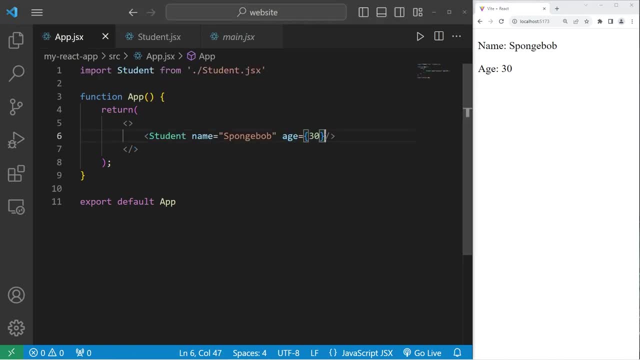 is 30.. Okay, let's send is student. Is Spongebob a student? We'll create a key of is student equals. add a set of curly braces. Is student will be a Boolean, true or false. Spongebob is in boating school currently. He is a student. 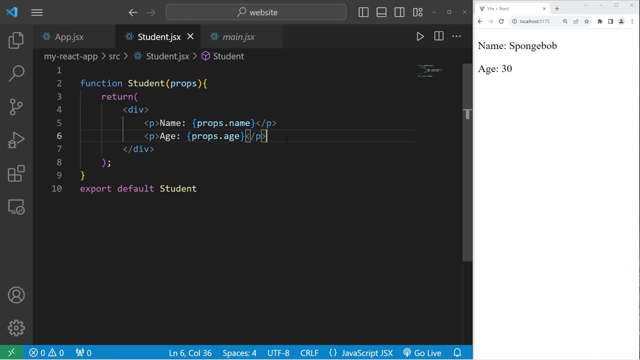 Let's save. Heading back to our student component, I'll include a new paragraph: Student colon space. curly braces props dot is student. Spongebob is a student, That is true. However, our Boolean is not displaying, So with a Boolean, I recommend using the ternary operator. 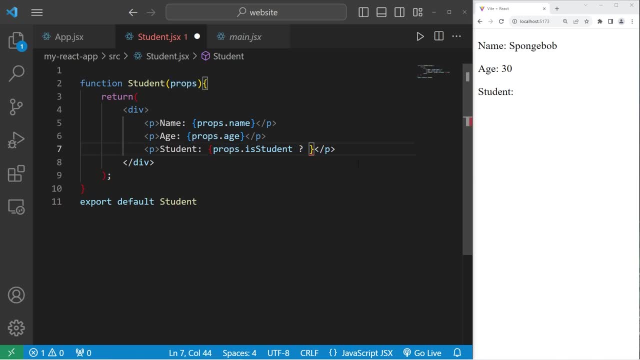 If is student within props is true, then we'll return a string literal of yes. Otherwise, we'll return a string literal of no. Let's update everything. Yes, Spongebob is a student. You can place complex JavaScript code within your HTML code. Booleans don't display. 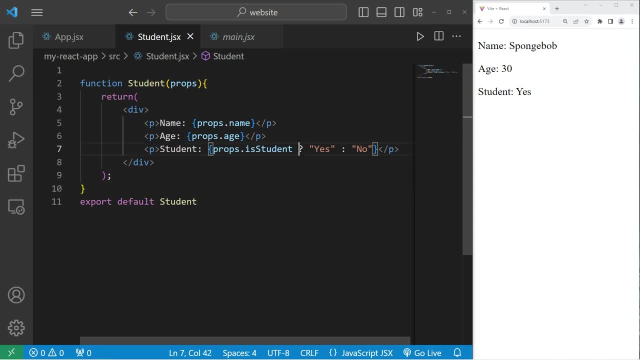 They're displayed directly to the DOM You find them used in Ternary Data Operators. If some value is true, return, or do this. If not, do something else. Now, if I were to pass in a Boolean value of false, well, that will change to no. Spongebob is not a student. 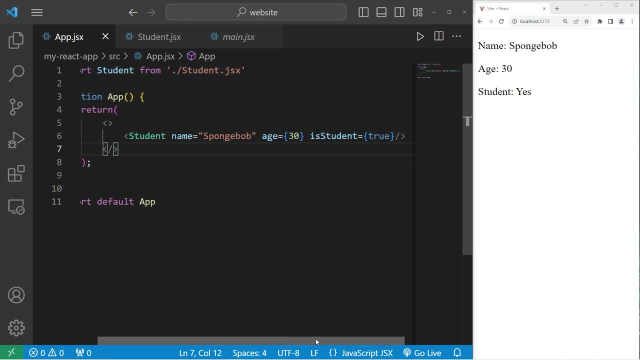 Let's change that back to true. Before I include a few more components, I'm going to do a little bit of CSS styling just so that all of this is going to be more readable. I'm going to zoom out to 100% where it was originally: Within my student component, within the enclosing div element. 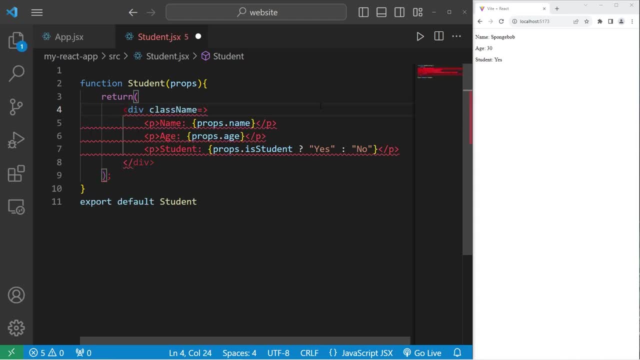 I will set a class name. Remember that with JSX you have to use class name, not class, because class is a reserved keyword. Let's name this class student. Then heading to our CSS stylesheet: indexcss. feel free to clear out anything within here. I will select the class of. 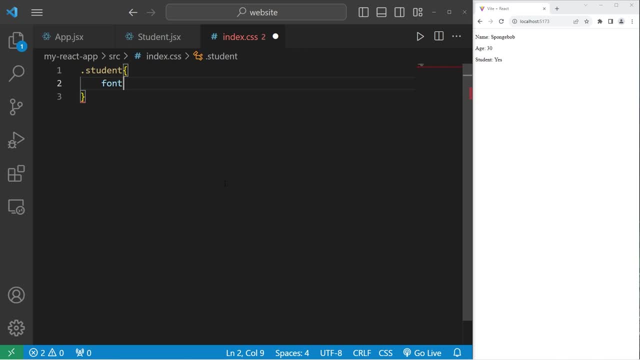 student. I'll change the font family to be Arial. I'll add a backup of sans-serif in case Arial can't display for some reason. Let's change the font size to 2em for 200%. I'll add a little bit of padding: 10 pixels. 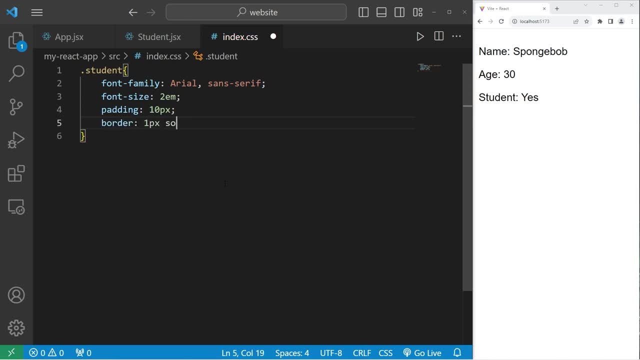 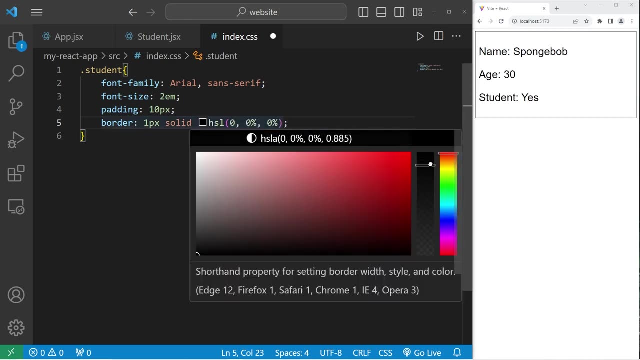 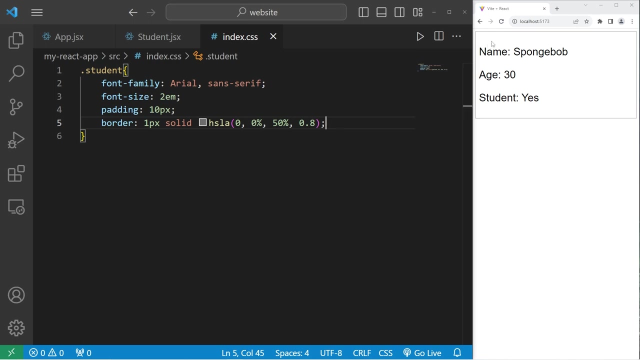 I'll add a border Border: 1px solid. Pick a color, I like HSL values. I'll set the transparency down a little bit, like 80%. Let's go with like 50% lightness. I'll remove any margin around the. 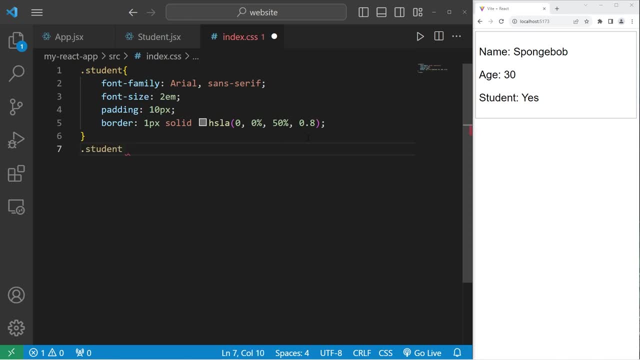 paragraph elements. We are accessing the class student. Then access any paragraph elements. Margin 0.. Okay, that's not too bad. So this is a student component to display some student data. We'll reuse the student component but pass in different data each time. We'll create a new student component. 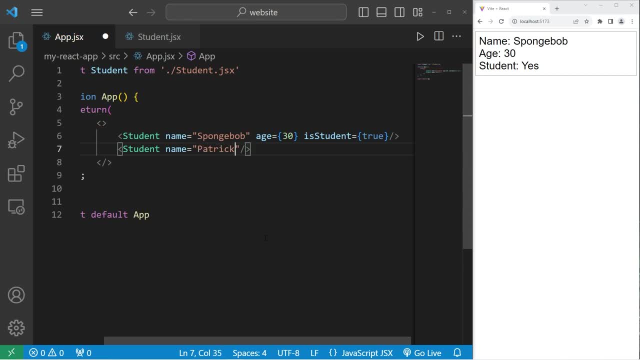 This student's name will be Patrick, Patrick's age. Patrick will be 42.. Is Patrick a student? Is student. I will set that to be false. Let's update our web application And there is Patrick's data Name: Patrick, Age, 42.. Student no. 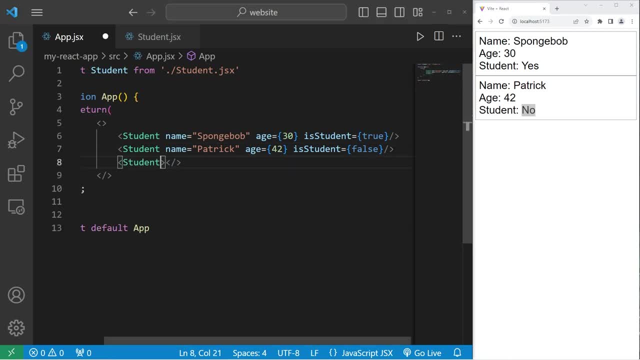 Let's add a few more. Student name equals Squidward. Squidward's age will be 50. Is student, Squidward will not be a student. That will be false. Then let's add Sandy. She'll be the last student. 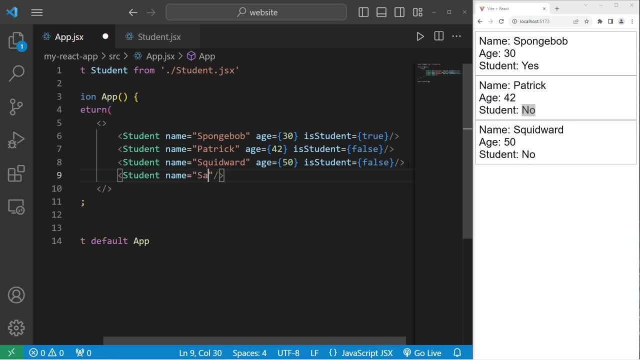 Student name equals Sandy. Sandy's age will be 27.. Is Sandy a student? She will be. That will be true. There we are All right. we have created four student components. Each has different values depending on what we pass into props. 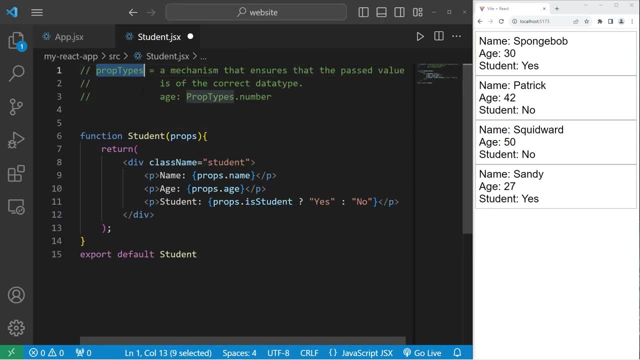 We're going to move on to prop types. Prop types, Prop types, are a mechanism that ensures that the passed value is of the correct data type. For example, within props we have an age. We would like to ensure that the age value passed in is a number, not a string or a boolean If it. 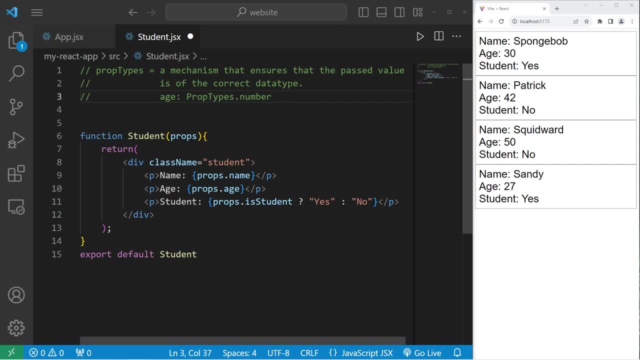 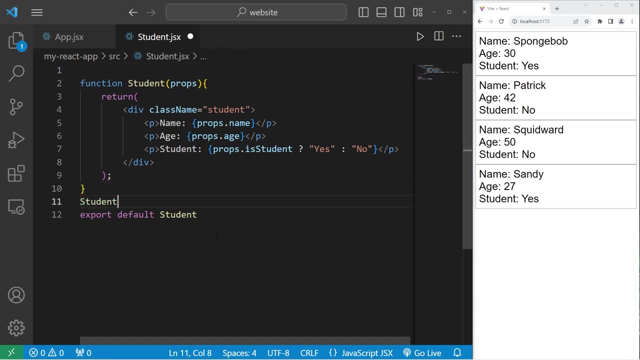 isn't, then React can emit a warning within our console, mostly for debugging purposes. If you're working with props, it is good practice to also use prop types, So here's how to create prop types. After our student function, we'll type the name of the component: student dot. prop types. 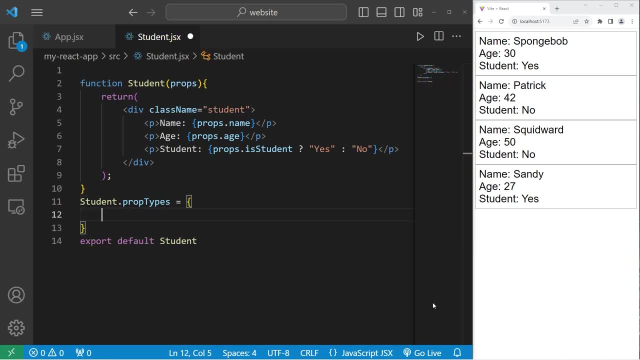 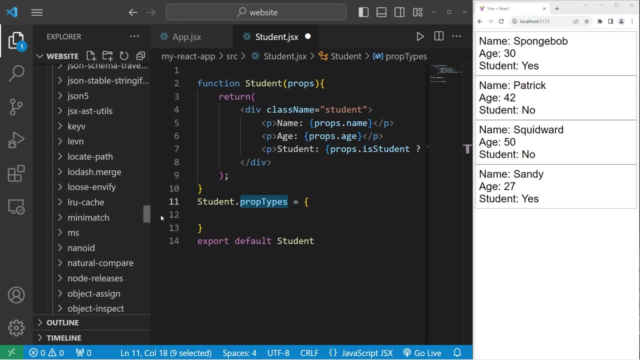 equals curly braces. Now we do have to import prop types. It's found within the node modules folder. Where is it? This should be in alphabetical order. There it is prop types. At the top of our JSR file we have prop types. If we type in prop types we do get to an alphabetic order. There it is, Prop types. I'll assign the alphabetic order And then I'll need to do a new read. My way of doing the read I'll need to do is into the Ref meet喝. That will be done. I've got a new read, so I'll add all the key words in the list. Then I'll add a new read to the list. 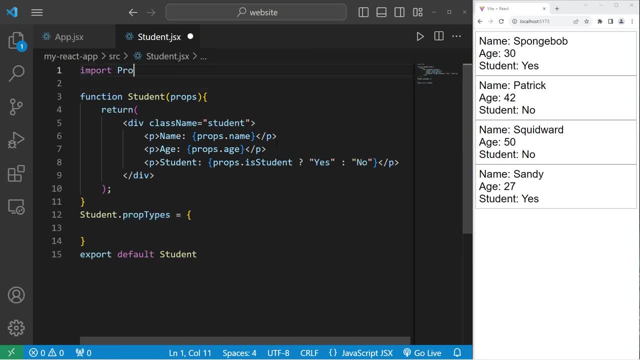 At the top of our jsx file. we will import prop-types from prop-types Within our prop-types. I would like to ensure that any name passed in is going to be a string. If it's not, we'll issue a warning within our console. 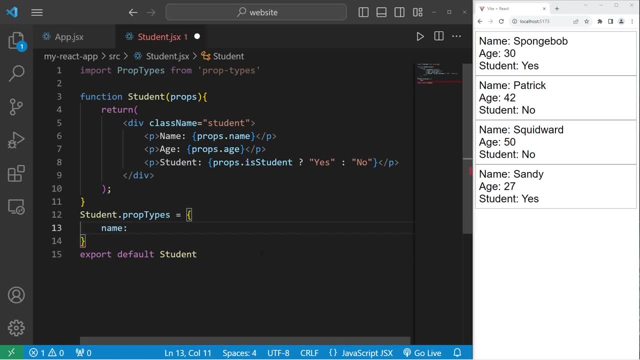 Name colon space Prop-typesstring. Age will be a number Age colon space Prop-typesnumber. Isstudent is a Boolean. Isstudent colon space Prop-typesbool. those are our prop types. Heading back to our app component For Spongebob's age, if I don't pass, 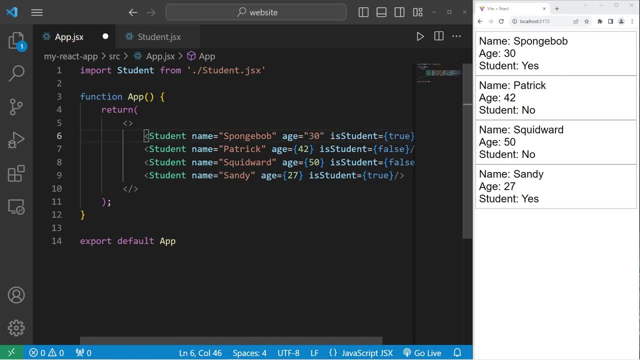 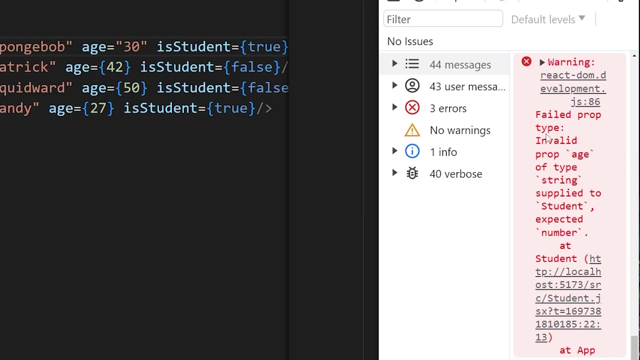 in a number. let's say I pass in a string, A string of 30. Well, this won't prevent the program from running, but it will issue a warning within our console. If we right click, go to inspect, go to console, we can see a warning: Failed prop type, Invalid prop. age of type string. 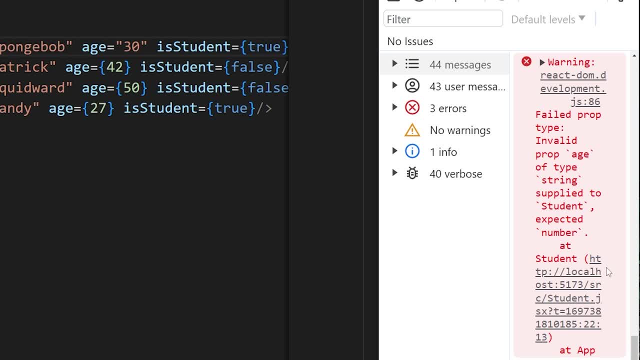 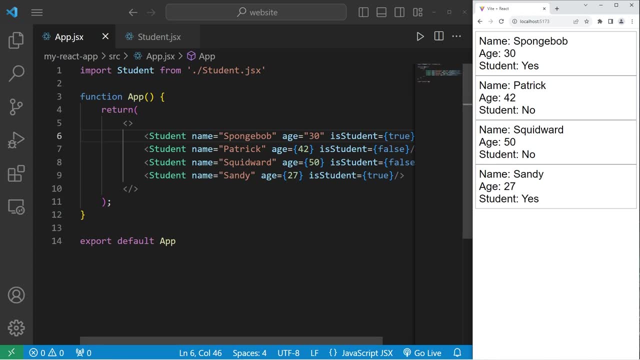 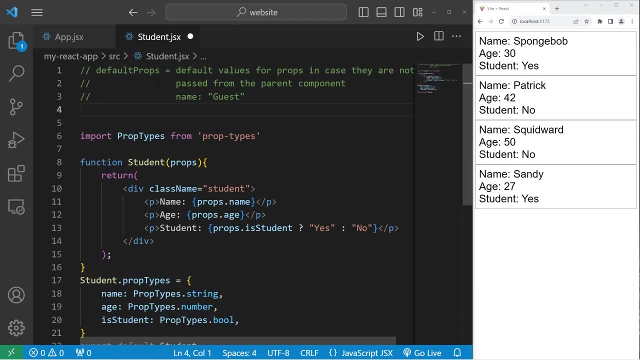 Supplied to student Expected number. And here's a location. So this is good for debugging. It won't stop the application from running, just issue a warning. It is good practice to include prop types. if you're accepting props, Then, lastly, we're going to discuss default props.